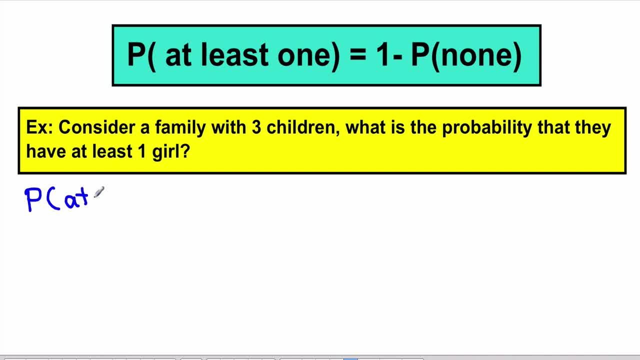 probability that they have at least one. So probability of at least will be 1 minus probability of no girls, which is basically 1 minus probability of all boys. now the kids being boy or girl are independent events, so probability of all boys will be for the first child being a boy is 0.5. for the 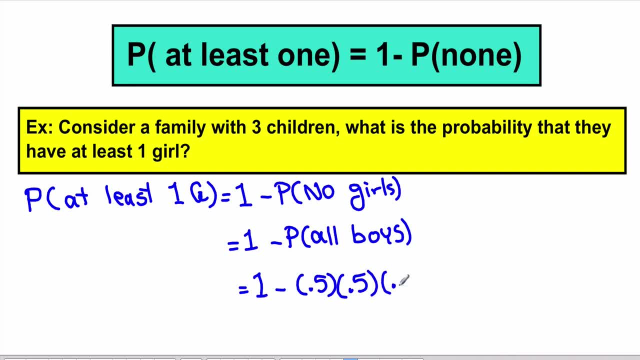 second child is 0.5 and a third child is 0.5. so we're using the concept of multiplication rule and the events being independent. once we simplify this, we get point eight seven five. so probability of having at least one girl in a family with three children is point eight seven five. now let's look at 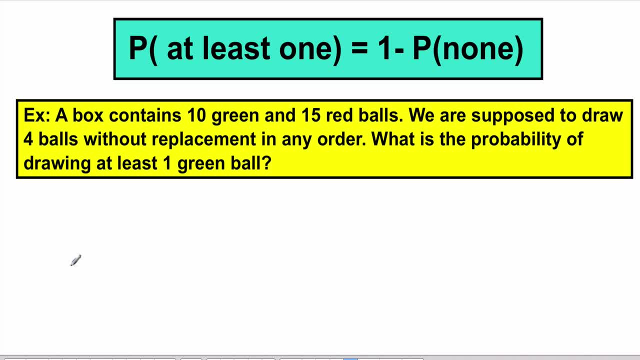 our second example. we're going to draw four balls and the question is asking: what's the probability of having at least one green ball? so once again, the keyword here is at least, and probability of at least one is going to be one minus probability of none. so this would be one minus probability of no green ball. 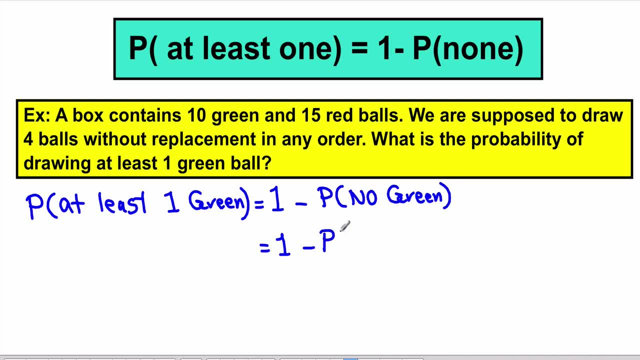 now, no green is the same as the green ball having probability of all red balls. now, altogether, we have 25 balls and we're drawing four balls. there are ten green balls available, but our desired event is all red balls, so we're selecting none of those green balls from the 15 red balls we're going to draw. 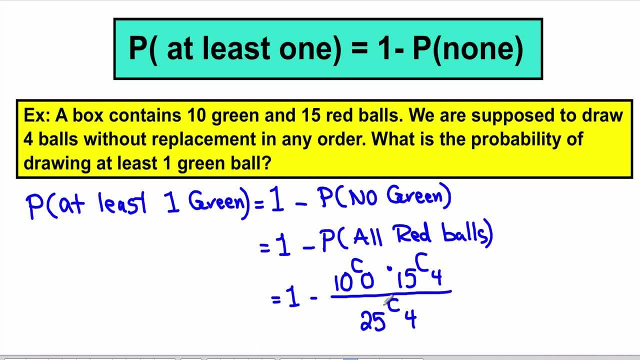 four balls. so once we simplify this, we're going to get 22, 57, over 25, 30, and if I play, put this in decimal, I get point eight, ninety two. so here probability of getting at least one green ball when we have 10 green balls. 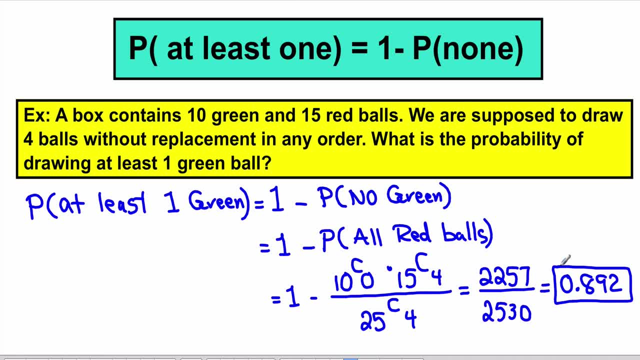 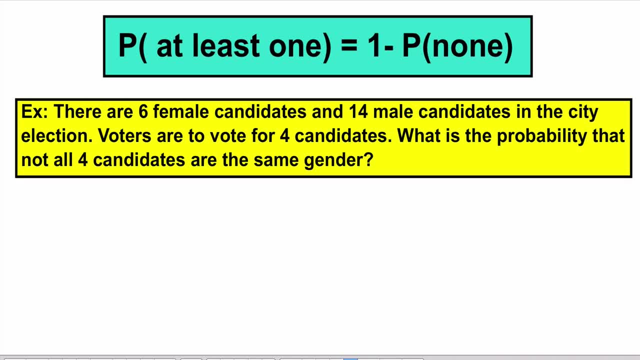 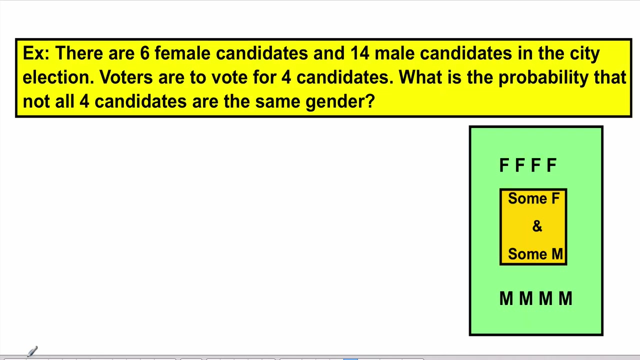 and 15 red balls and we're drawing four balls is point eight, nine, two. now I consider a election with six female candidates and 14 male candidates, and all voters are supposed to vote for four candidates. we want to know what's the probability that not all four candidates are the same gender. well, it is possible that we get. 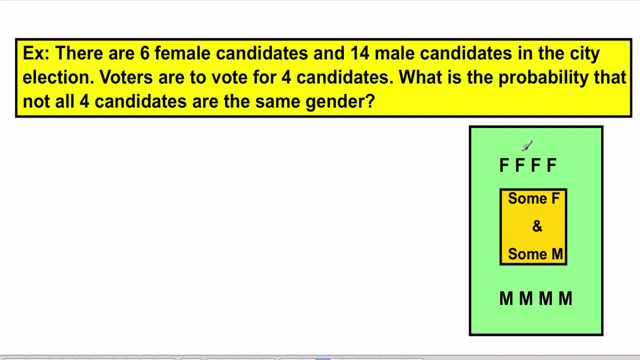 all four candidates to be females. it is also possible to get all four to be male, but these are not the desired event. the desired event is that, all four candidates not having same gender, so we want some female and some male, so probability that they are not all same gender.